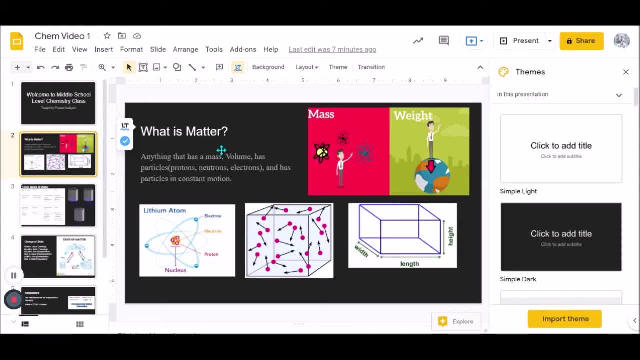 mass volume and has particles- Protons, neutrons, electrons, and here's a model- And has particles in constant motion. Here's a misunderstanding, which is people confuse mass with weight. Now, mass and weight are different things, because mass is the amount of matter in something, Now weight. there's a formula for weight which is: 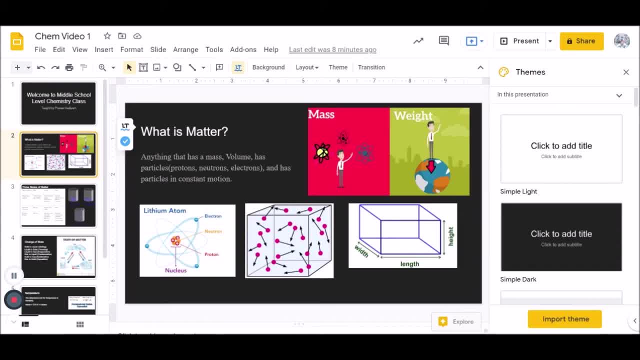 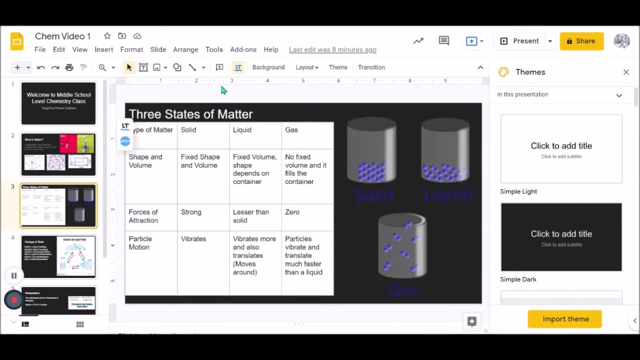 weight equals to mass times gravitational force. So that's going to be, that's going to be. quite it's not going to be the same because it's being multiplied by the gravitational force. Okay, let's go on Now. there are three states of matter. There's solid liquid. 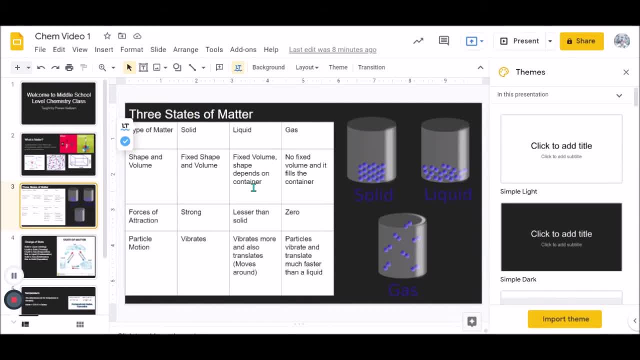 and gas and each have different properties. Now, a solid has a fixed shape and a volume. As you can see, it's all connected properly. and liquid, on the other hand, it has a fixed volume. yes, the shape depends on the container. See, it's spreading out to the container. 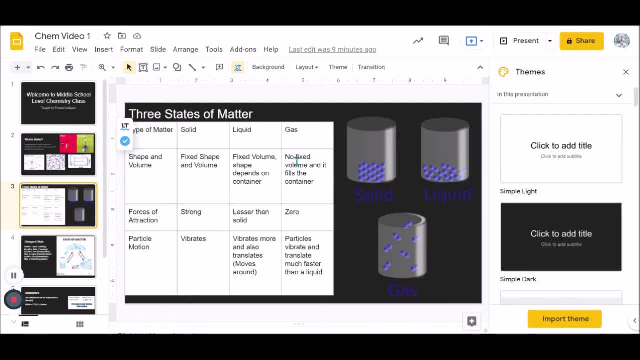 See that Okay. and then, lastly, gas doesn't have a fixed volume and it fills the container. It's more spread apart in the container. Now, in solid, the forces of attraction, The forces of attraction in solid, is very strong, and what I mean by that is: 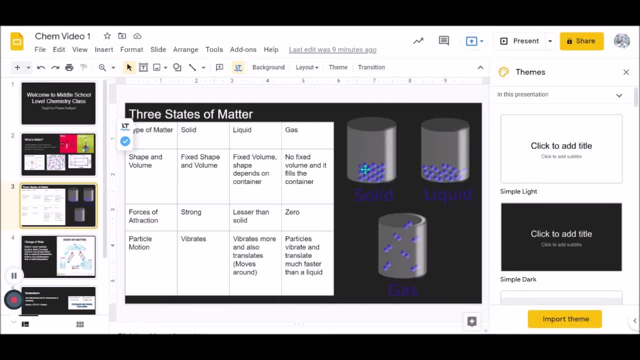 attraction between the particles. See, they're all connected very well. and then you know, as you go on liquid, the force of attraction becomes a little weaker, and for gas we come to the zero because it spreads apart. Okay, now particle motion. Now, in solid, the particles are actually vibrating. 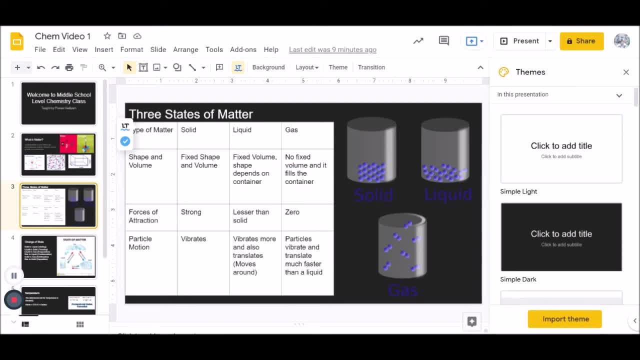 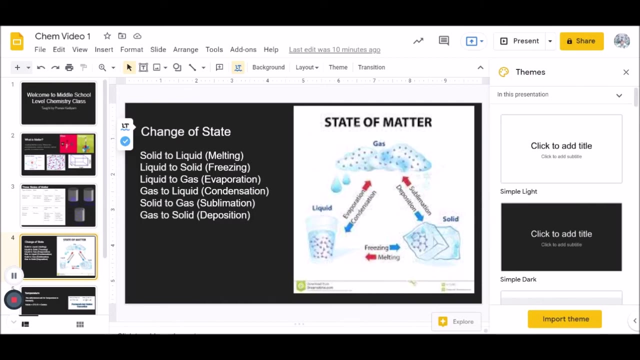 Okay, as I said, in all matter they have to have a particle that's in constant motion more and it also translates, moves around. okay. and for gas the particles vibrate and translate much faster than a liquid. changes in minutes, changes in states. now solid to liquid is called as melting and liquid to solid is called freezing. and 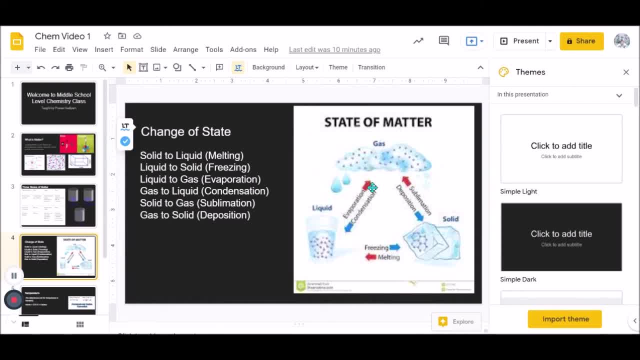 liquid to gas is known as evaporation and gas to liquid is. it is condensation and most most likely you have heard these terms when learning the water cycle: condensation, evaporation, transit, precipitation, all those stuff right. and then solid to gas is known as sublimation. example: solid to gas with 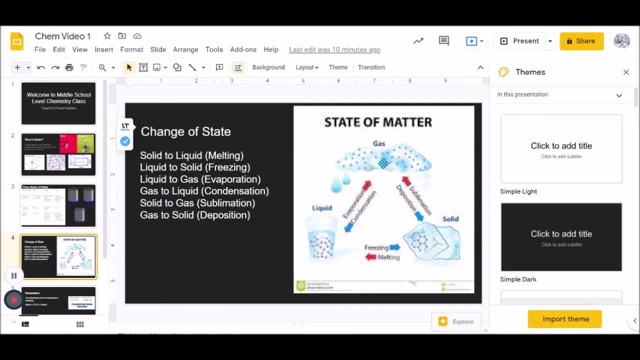 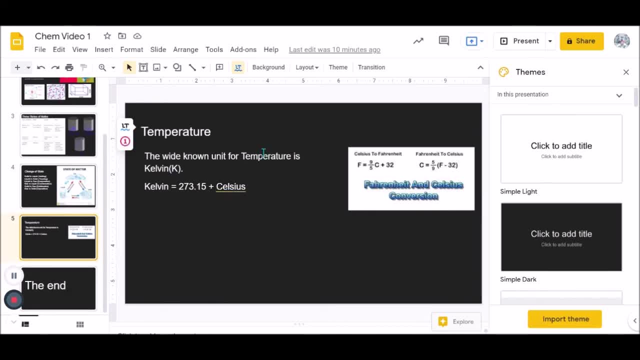 the dry ice and gas solid is deposition, and the topic of this video is a lot of stuff like this, but, for example, I saw some visible one that I've been looking for a lot of examples where it was a pretty off. this is the last part of our lesson for today. um, okay, so temperature. what is temperature exactly? 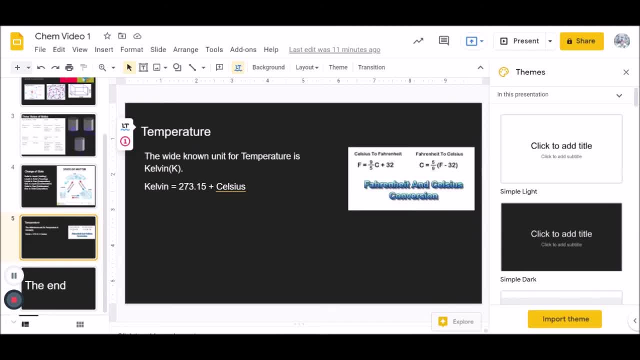 temperature is used to measure the like we are not really sure about. like, for example: um there's this ice and there's this, um hot chunk of, let's say, magma or something. we use temperature to measure how, how hot or how cold something is okay and um. the wide known unit, or the si unit for temperature is kelvin, and here's the formula. 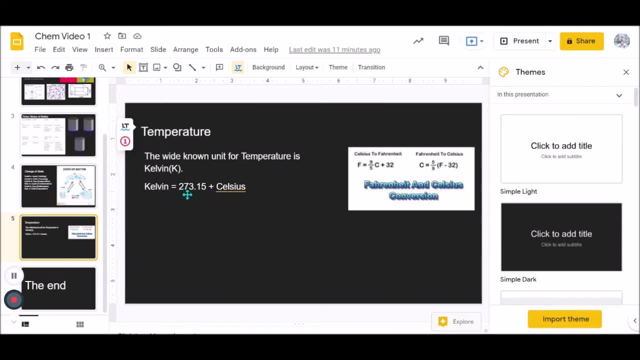 for kelvin. kelvin is equal to 273.15 plus celsius. now most likely, uh, when. when you hear temperature, you always think of celsius or fahrenheit and um but um. but when it comes, when? but when you get to higher levels, you should make sure that you use. 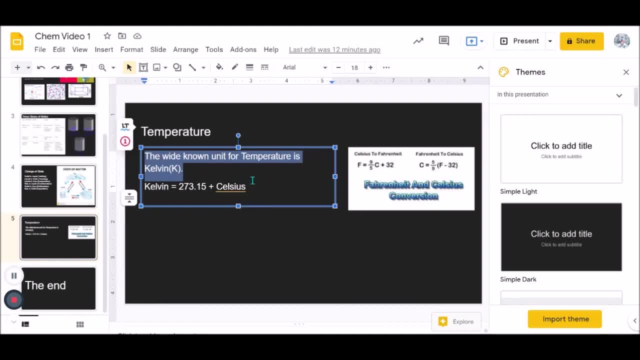 kelvin. well, i mean, it depends on the um, the unit they're asking for, but people prefer kelvin. i believe so and um. if you would like to convert the celsius and fahrenheit, here's the formulas. okay and um. thank you for listening. i believe that's it. 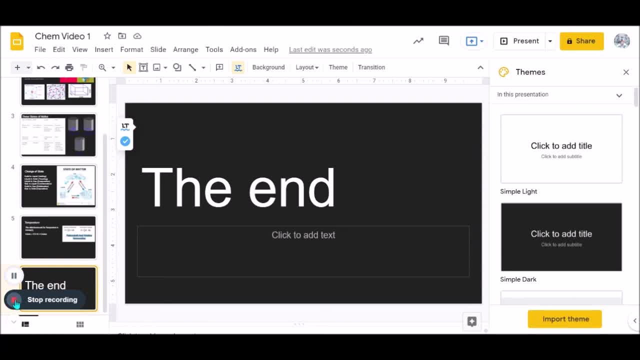 um well, i hope i get good results. thank you, goodbye.